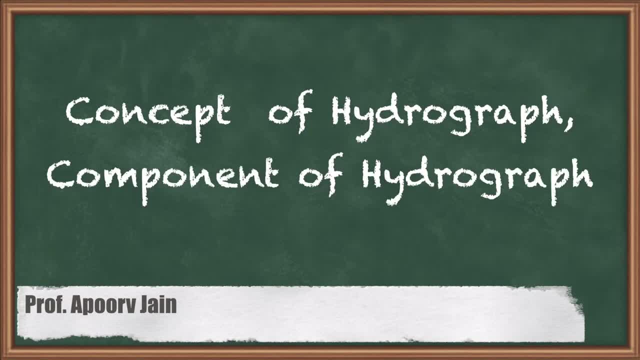 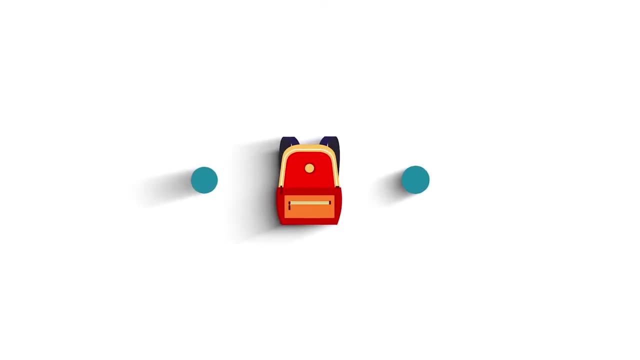 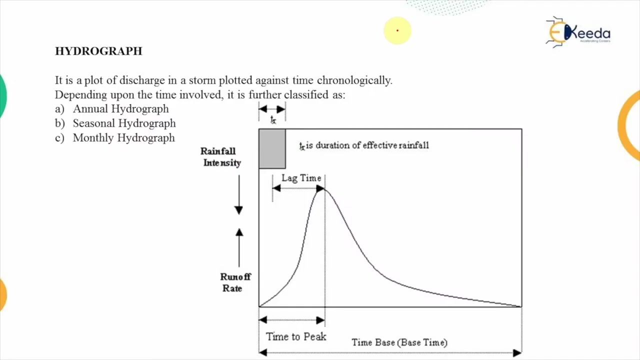 Hello everyone, In this video we are going to discuss about the hydrograph, which is used to represent the rainfall occurring in a particular catchment area, and then what are the components of the hydrograph. So let's start. So, first of all, what is a hydrograph? So it is a plot of a discharge in a storm, plotted against the time. chronologically, That means, let's say, the rainfall started with the zero hours. So for the first hour there was certain volume of the rainfall that has occurred and let's say we are 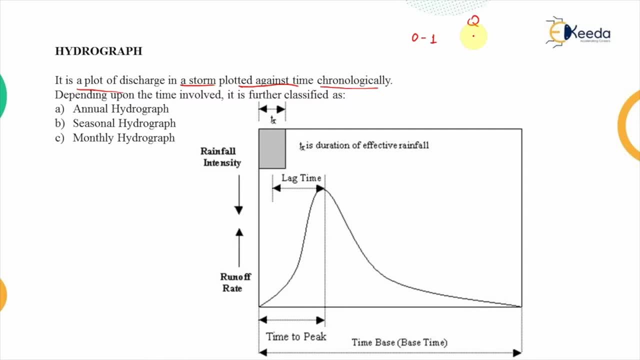 taking the random values for the discharge in that time period. So for the first hour the discharge was 10.. For the next hour, that is, for 1 to 2 hours, the discharge increased and that has reached up to the 15 value. For the next 1 hour, this value further increased and it reached up to 20.. So as the time progresses, the discharge will keep on increasing. 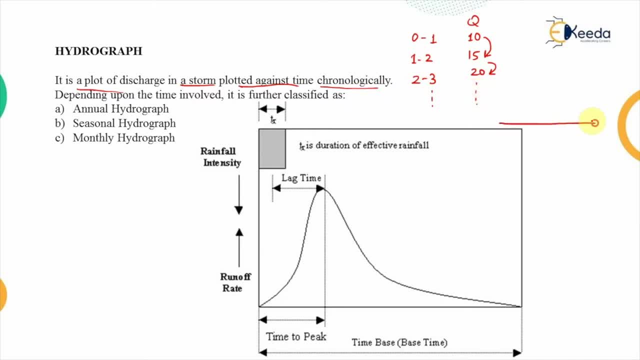 So let's start. So the reason behind that is for the particular catchment area when the precipitation is happening, when the rainfall is occurring. in that case, initially the rainfall which is occurring in a catchment area, that will be accumulated and it will be moving over the surface after a while. So initially there is a lesser flow, but once the rainfall is constant it will increase. 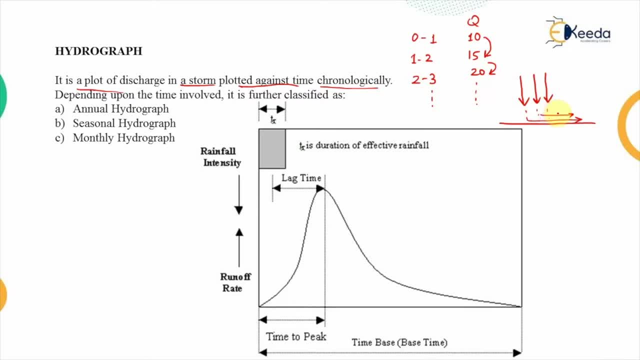 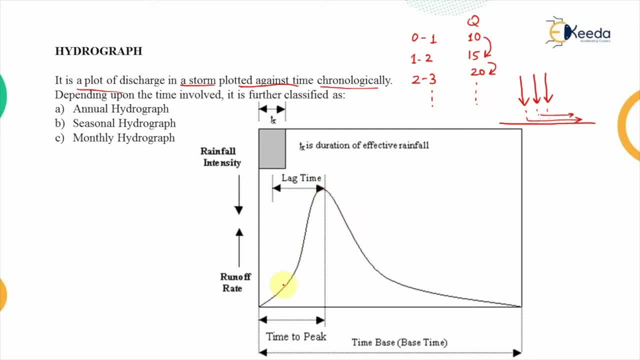 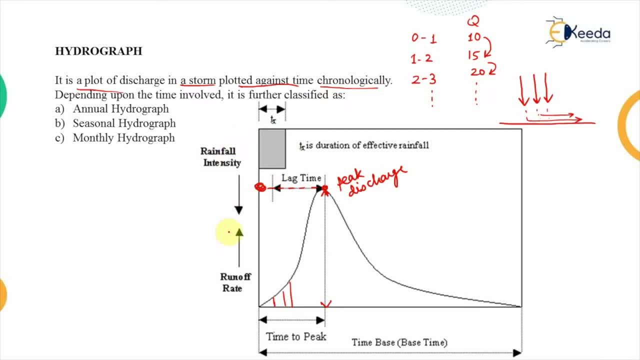 This y-axis is representing the runoff and the x-axis is representing the duration, Assuming that the curve started from the 0 hours. so the time taken to reach to the peak discharge, that is known as the time to peak, And the entire time period which is taken by the hydrograph, because once the rainfall has stopped, but the water which has been collected during that rainfall, that will still be present and that will take enough time to move out of the catchment area. 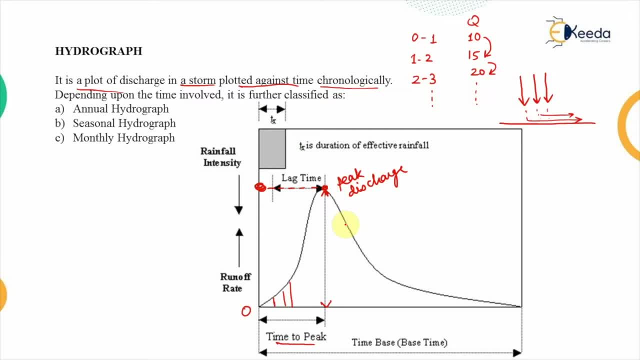 So that's why the curve will start decreasing. there will be a fall in the curve, but that will be very slow and ultimately we will get the 0 point again. So that will mark the completion of the hydrograph and the completion of the storm. 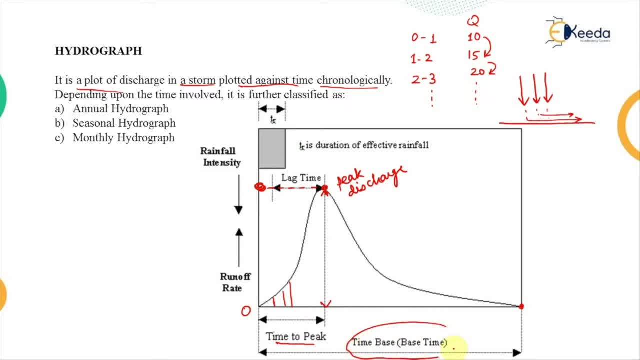 So this time period which is representing this, is known as the base period or the base time. Correspondingly, we are having this hydrograph here that is representing the rainfall intensity, So we know that the effective rainfall that we are considering that is usually 1 cm. 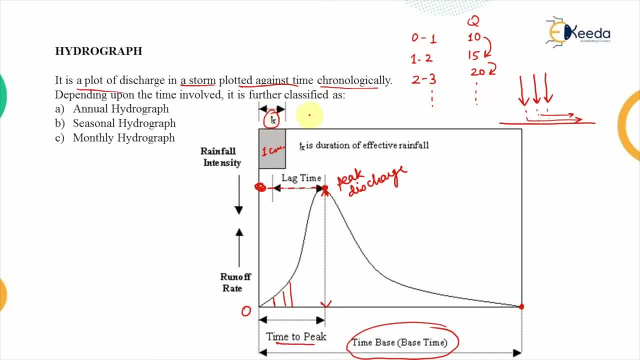 And that is occurring For the TR duration. so the rainfall intensity is usually 1 cm divided by the time period and that will be in cm per hour. So that will represent the rainfall intensity. Now, depending upon the how much time is involved in the particular storm, it is further classified according to that. 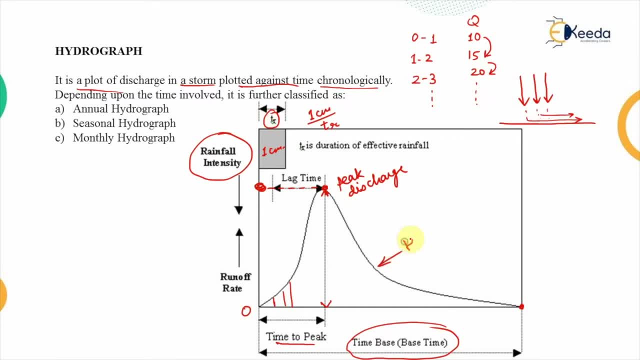 So this curve that we are getting, that is known as the hydrograph And that is classified according to the time involved. So if the entire data is collected, corresponding to the entire year, then the hydrograph that we will be obtaining for that storm is known as the annual hydrograph. 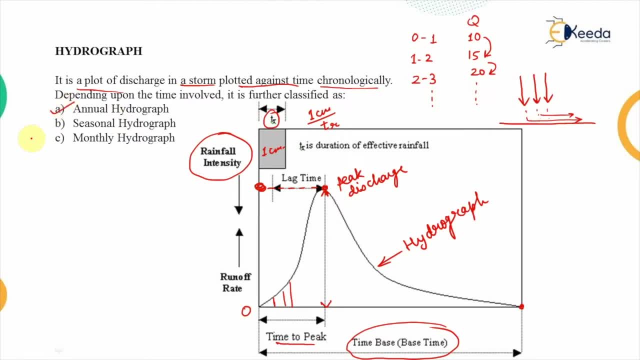 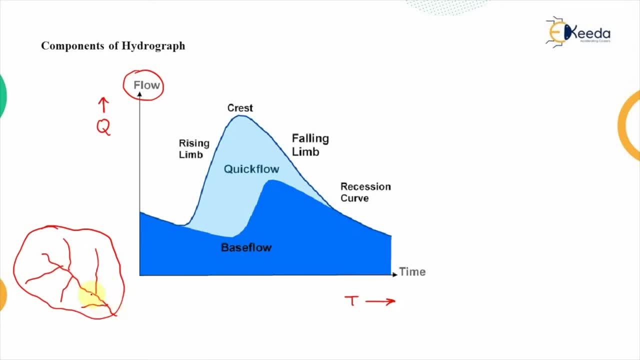 towards it. So we will take a point which is exiting the catchment area, So we can say that this is the point that I am marking, that is the outlet point, and so we will write that. Now there is a particular term that is involved with. 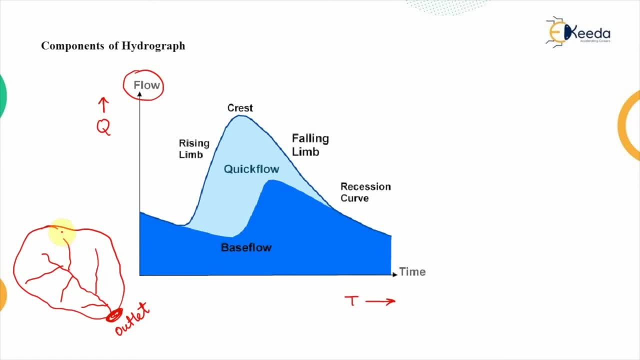 the time taken by the water from the remotest point or from the farthest point. that means the point which is situated at the maximum distance from the outlet point, the time which will be taken for the water droplet to come from that point and to reach the outlet. that particular time period is known as the 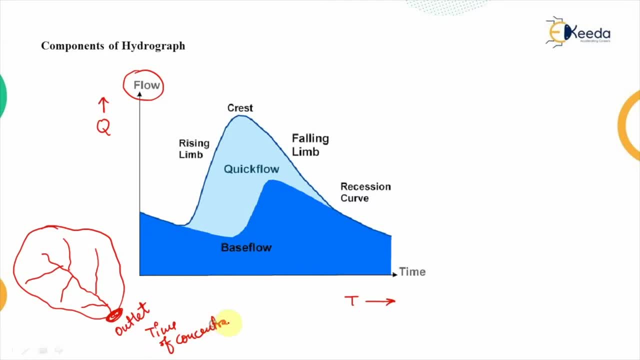 time of concentration. So usually that is the maximum time which would be taken by the water droplet and that is usually equal to to the base period that we represent by Tb. so because the ultimately the water droplet that is at the maximum distance, that will take the maximum time to reach. 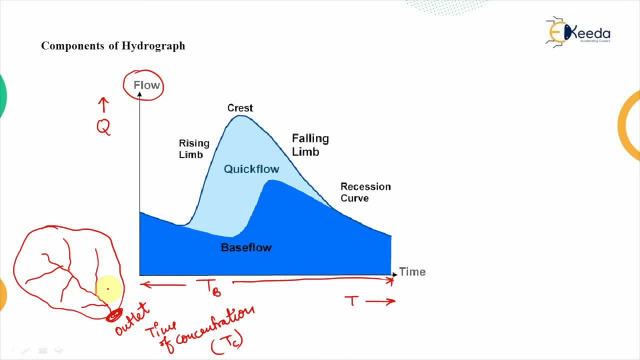 to the outlet. now, what are these components? so, when the water is flowing, when the precipitation is happening, so initially, for a minute time period, there is a decrease in the flow. the reason behind that is the maximum flow that is occurring that is not falling or that is not moving over the surface. that is. 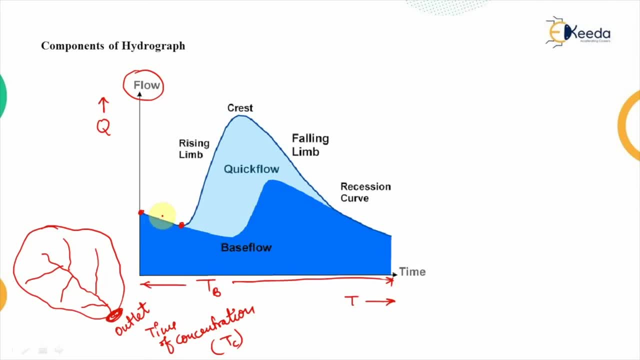 going inside the surface and that is why this segment- let's say we are denoting that as OA- so this OA segment that is representing the base flow. what is this base flow? base flow, So we have seen that the runoff which occur on the surface, that is a composition. 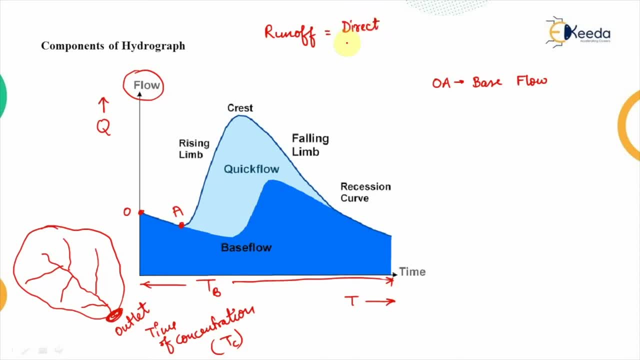 of two of the values, that is, the direct runoff, that means the runoff which is occurring on the surface, and the base flow, that means the flow which is occurring in the ground. So the component of these two, because ultimately the runoff will be because of these two factors. 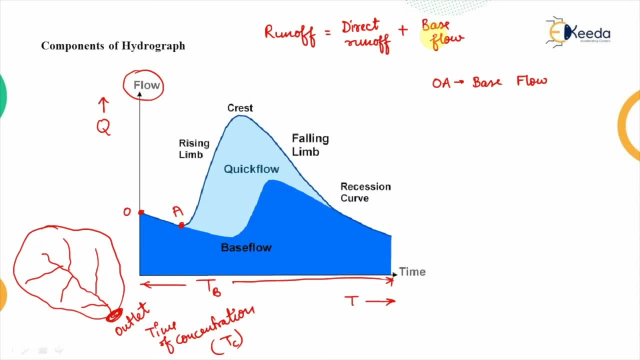 So the first component is the base flow, which is the reduction. So that is why this segment is known as the base flow recession. The next segment, as we can see, is the rising part or the rising segment of the hydrograph. Let's say this point is b, so this: is is b here. so this is b here. so this is the rising component of the hydrograph. so lets say b, this is the rising component. почему we are discussing about. so, as you will understand by the start of this phrase, here, for this paragraph the sample is negative. Before we 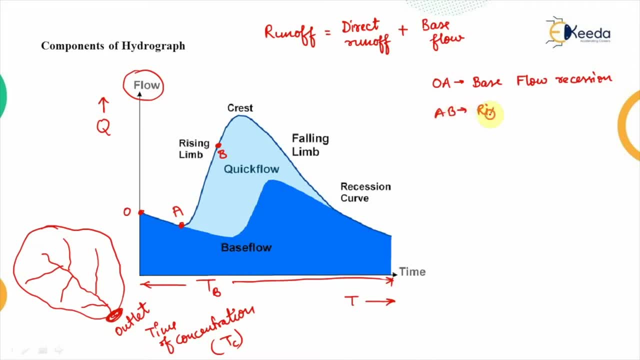 B segment that is known as the rising limb or the rising segment. corresponding to this, we will mark the similar point on the other side, from which we can say that the curve has started falling, and this segment between these B and C point that is known as the crest segment or the peak of the hydrograph. 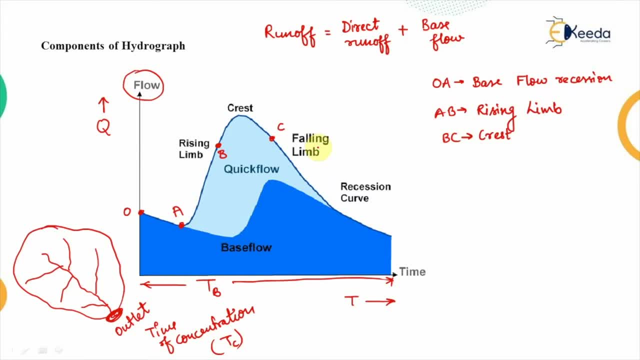 now, when we reach the point C, it has been observed that the curve is starting to decrease. so from that point and till the point the base flow is contributing, that segment is known as the falling limb or the receding segment- and again after that, as we were obtaining the initial part of the hydro curve, 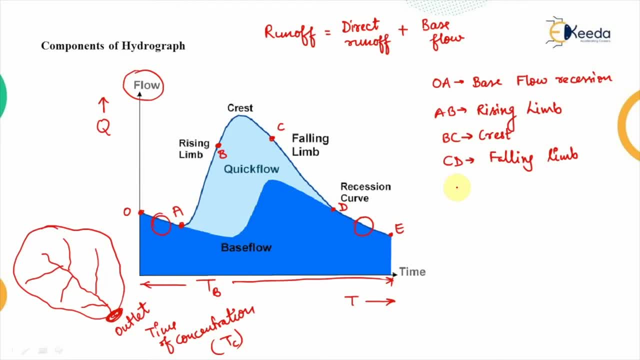 we will mark the same point on the other side and we will mark the same point on the other side as we were obtaining in the initial phase of the hydrograph. the same segment is obtained where the base flow is reducing because the contribution towards the runoff is from the 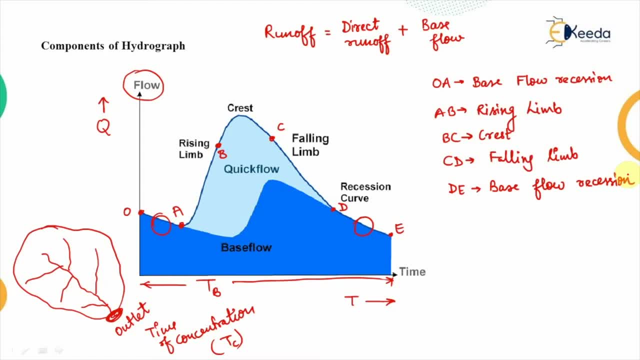 base flow, and that is why this segment is again known as the base flow recession. now, in this point, the curvature is also important. so we have seen that the maximum discharge we are getting, corresponding to the peak value, is known as the peak discharge and is represented by Qp. Now the curvature for the rising limb and the falling limb, both of these curvature. 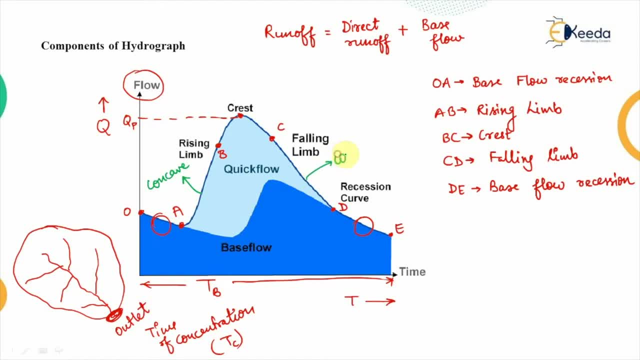 are concave in nature. This is also concave and this BC portion and the nature of this BC portion, that is convex because that is outwards, is convexity- is present. Now the points where this curvature is changing, that is a mathematical term. So the point where 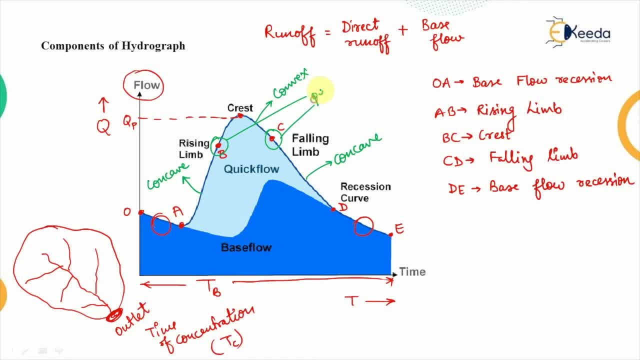 this curvature changes. that is known as the point of inflection. So, corresponding to a hydrograph with a singular peak, we will obtain Qp. If there are number of peaks, then the point of inflection obtained will be corresponding to that. Similar to these terms, there is one more term. So when we plot the hydrograph, 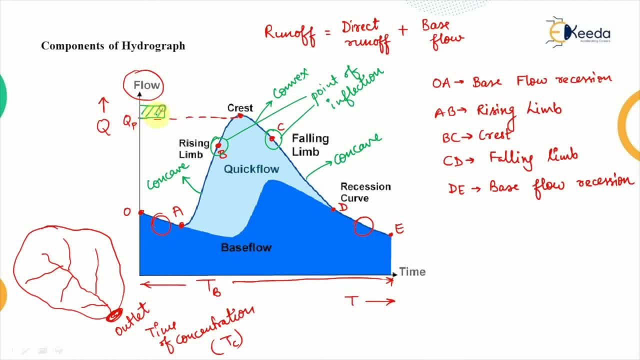 this hydrograph is obtained here. That is representing the rainfall. So rainfall is for a shorter duration, The storm occurs for a lesser duration, but the implication of the act that is obtained in the form of the runoff that is evident for a longer duration, That 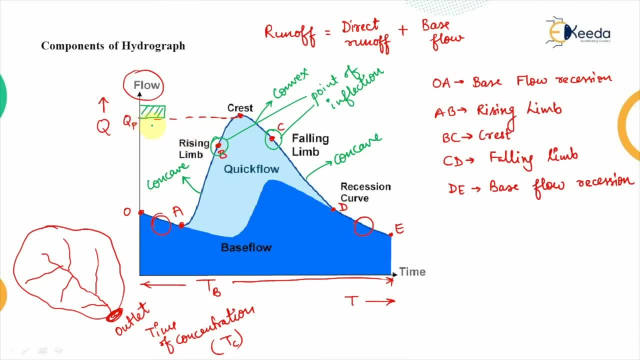 is why this hydrograph will be for the shorter duration. So, from the centre of this hydrograph, the distance of the crest of the, from the centre of the hydrograph to the peak of the hydrograph, the duration which is taken here, that is known as the time lag or the duration. 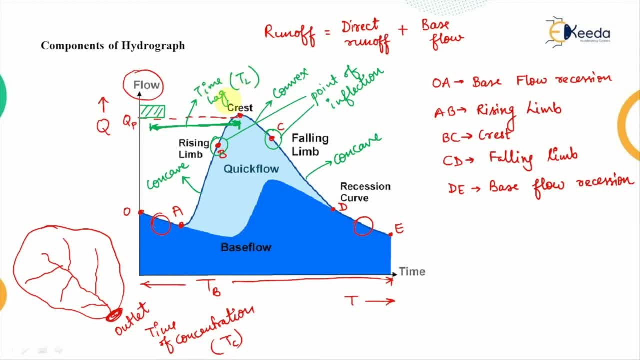 So in this case, this is the time lag that is represented by TL. Now, this completes all the components of the hydrograph. Now there are different factors which affect this particular shape of the hydrograph and broadly we classify these factors in two categories. that is, the 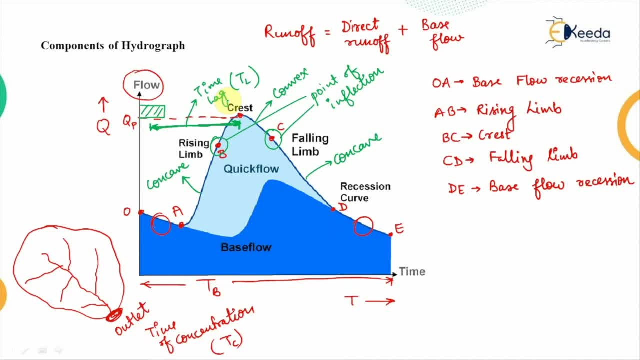 climatic factors and the geographical factors. So, one by one, we are going to discuss that what we are going to do in this hydrograph, So we are going to discuss that what we are is the implication of these factors on the shape of the hydrograph. so the first one is the climatic. 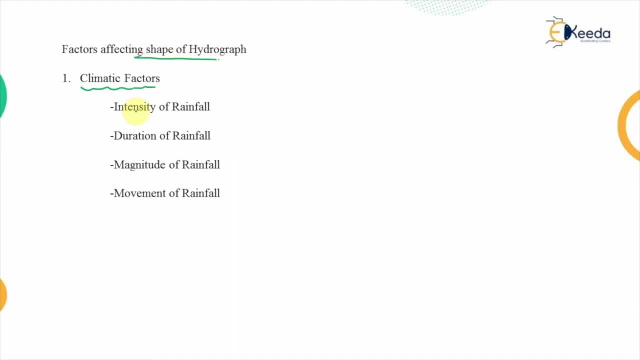 factors which affect the shape of the hydrograph. so first one is the intensity of the rainfall. now, if the rainfall is intense, if the rainfall is intense, then obviously the rainfall that is occurring that will be at higher magnitude. so in that case, initially the curve that we were 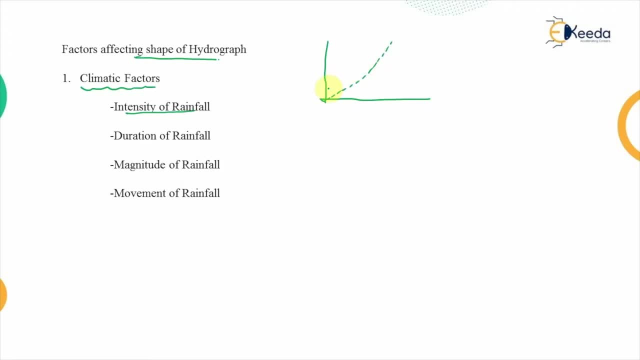 getting. this was the rising limb. so now we will be getting the steeper value of the rising limb because more runoff will be obtained in the shorter duration because of the higher intensity. so that is corresponding to the higher intensity and we will be getting the steeper rising limb, so that means this intensity of the rainfall, if that is. 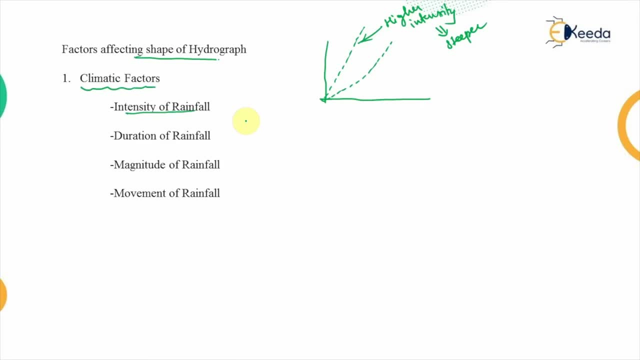 high is having an impact on the slope of the rising limb. similarly, duration of the rainfall. so if the duration of the rainfall, if that is more so, this storm that we will be getting, that will be also for the longer duration and because of that there is enough contribution from the stream, that will be for the. 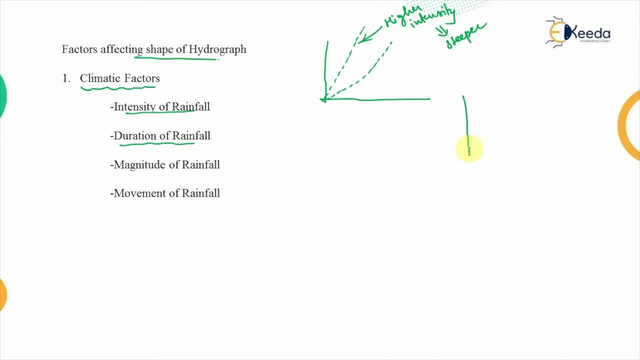 longer duration. so the curve that we will be getting, that is the hydrograph that will be having the more wider base. that means this base period will be increasing. if the duration of the rainfall is increasing, then the magnitude of the rainfall that will be again the same. 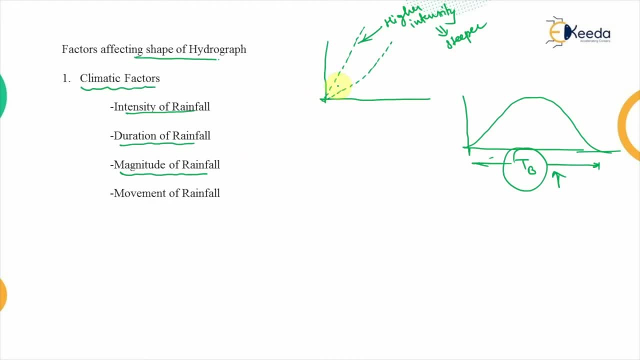 that will again be the same as was the first case, that in case of the magnitude increment, the curve that we are getting corresponding to the rising limb. that will be steeper, and then the movement of the rainfall. that means the runoff. so if the runoff is contributing early, if the movement is, 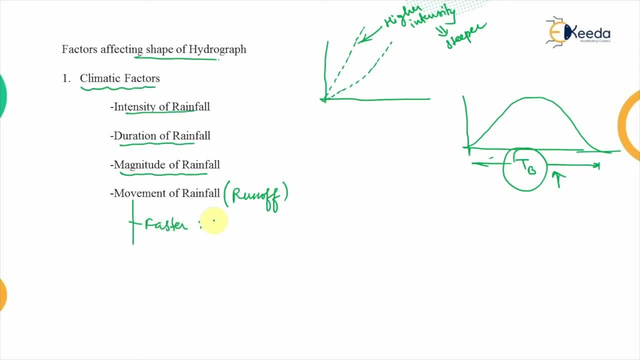 faster, then the peak that we will be obtaining that will be quicker and the steeper curve will be obtained because initially the contribution towards the outlet point that will be very fast and on the other hand if this movement is slow, then the peak that will be obtained that will be at a later stage. 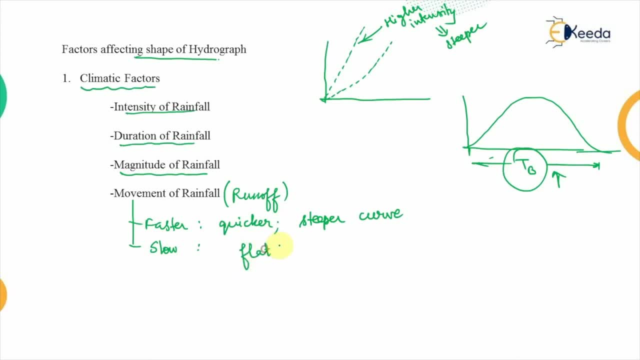 and the curve that we will be getting that will be relatively flatter. so if the faster movement is there, then this curve will be something like this and if we are obtaining the slow peak, then this will be the curve that we will be getting. So that is the impact of the climatic factors. 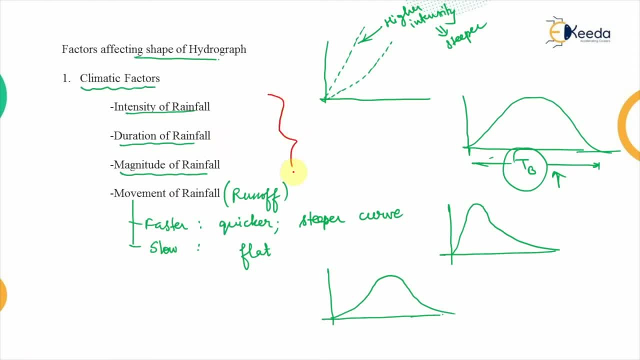 Now, in total, all of these factors are having majorly the impact on the rising limb of the hydrograph and not on the other segments of the hydrograph. Then the next category of the factors which affect the shape of hydrograph, that is classified as the geographical factors. 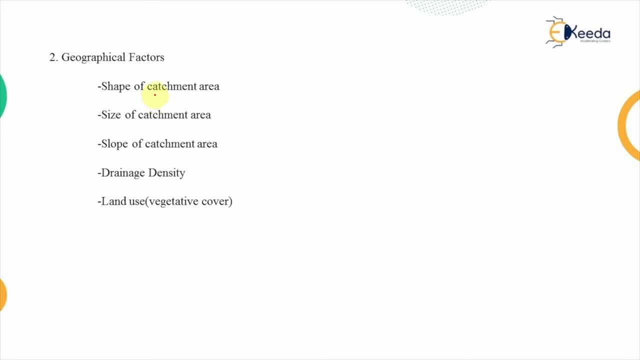 which are important ones. So, first of all, is the shape of the catchment area. that is very important aspect as far as the hydrograph is obtained. So, in total, all of these factors are having majorly the impact on the rising limb of the. So, in total, all of these factors are having majorly the impact on the rising limb of the. 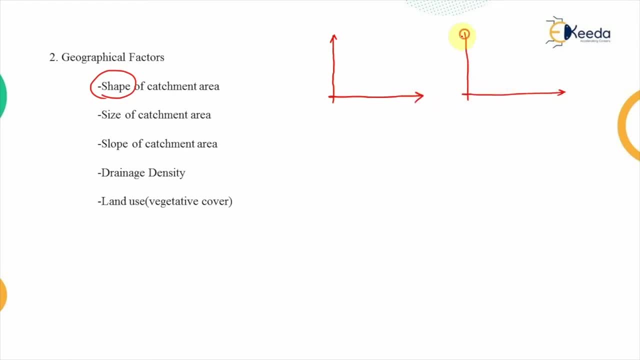 hydrograph. So we will obtain the hydrograph for the different shapes of the catchment area. So I am plotting these four types of the shapes of the catchment area, corresponding to which we will be obtaining the different hydrograph. So this first shape that is known, 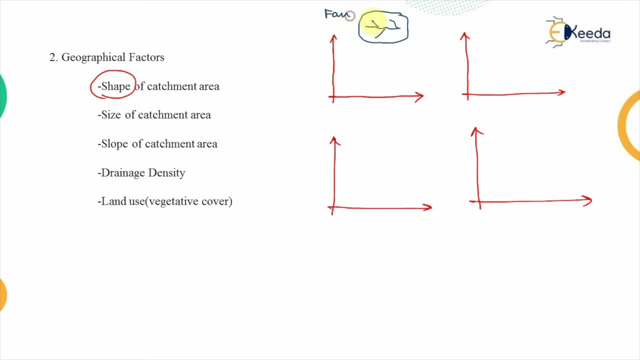 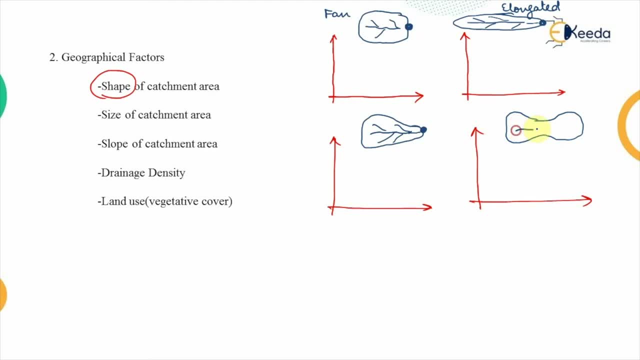 leaf with the two of the broad areas, so that is the another. Now, corresponding to all of these, we will be obtaining the different shapes of the hydrograph. so starting with the first one Now, this will be the plot between the discharge and the time, so we will be getting this as the shape of the 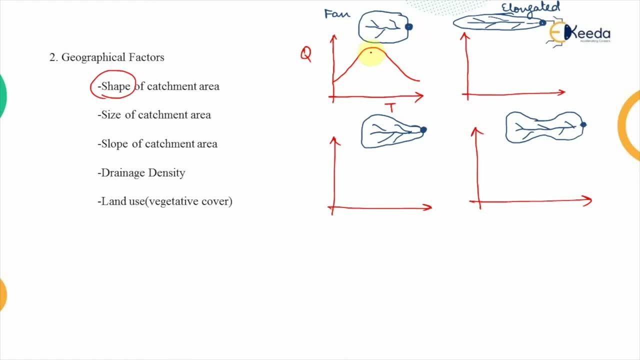 hydrograph. Now, the time taken by the curve to reach to its peak, that is the time to peak, that is Tp and that is the standard value of the hydrograph. that is the standard shape of the hydrograph that we obtained for the fan shaped catchment area, Because the contribution from each 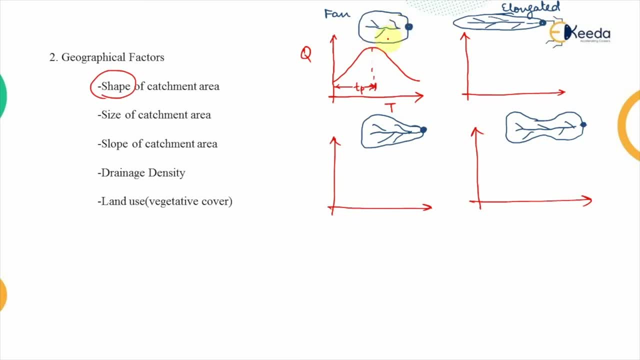 of the point towards this stream, that will be at the almost the same time. but if we take a look at the elongated catchment area now for this remotest point to reach to the outlet, that will take the maximum time. similarly, the points which are near to this remotest point, that will also take a. 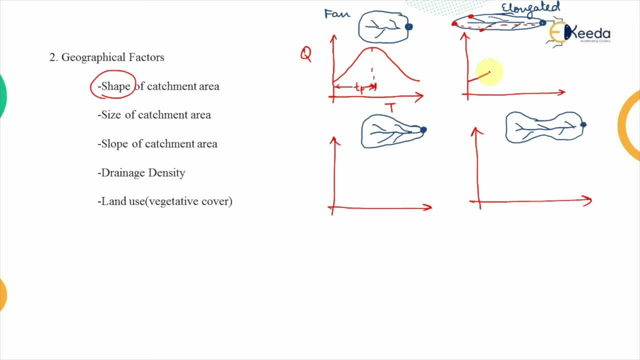 very huge time. so, because of that, this curve that we obtain, that is usually flatter and this is the time which is taken to peak the hydrograph. so, in comparison to the fan-shaped hydrograph, in comparison to the hydrograph which are obtained for the fan-shaped catchment area, the 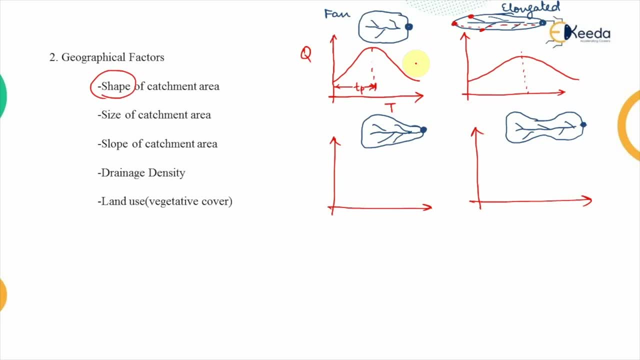 hydrograph for the elongated catchment area are flatter because the time taken by the water droplets to reach the outlet point is more shorter then if we are having this narrow leaf, so the points which are situated near to this outlet point that will be taking lesser time to reach this. 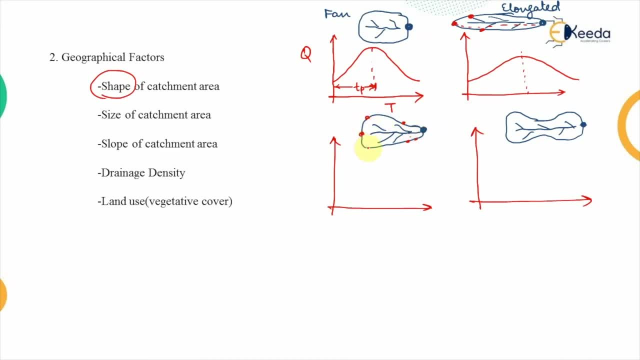 point, but the points which are at the farthest distance, they will take the maximum time and because of that, the peak that we obtain that is slightly shifted and there is some skewness in the curve and the shape of the hydrograph that we obtained for such type of the catchment areas. 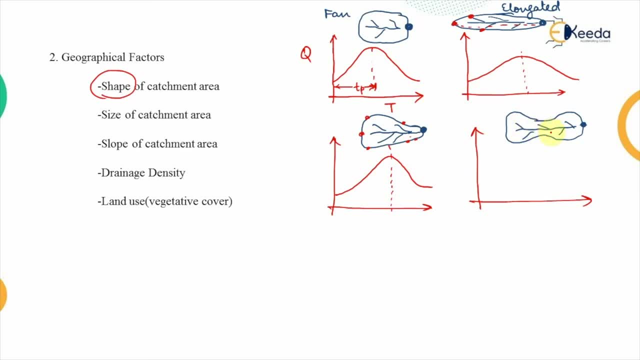 Then, similarly for this shape of the fourth shape of the catchment area, the first part of the catchment area will be contributing towards the outlet point quicker than the contribution from the back side and because of that the shape that we get for such type of catchment area. 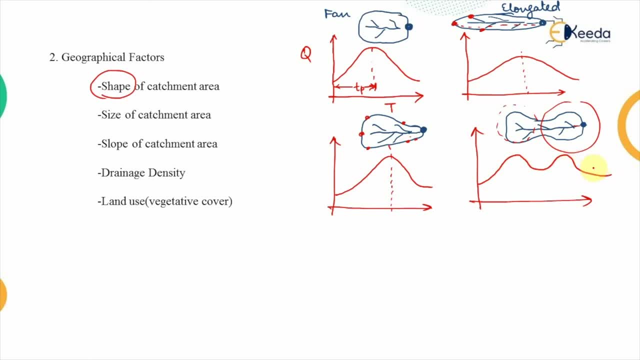 is involving the two of the peaks for the hydrograph. So this is the impact of the catchment area. There may be more number of the catchment area which may be available. so all of those plots of the hydrograph, they are obtained in the similar manner. The next factor is the 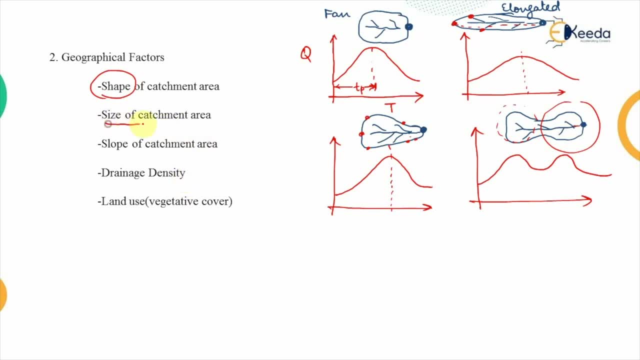 size of the catchment area. So if the size of the catchment area, if that is bigger, then obviously the peak that we will be getting that will be at higher discharge. So, for example, if let's say this is the hydrograph that we are obtaining for catchment area, which is 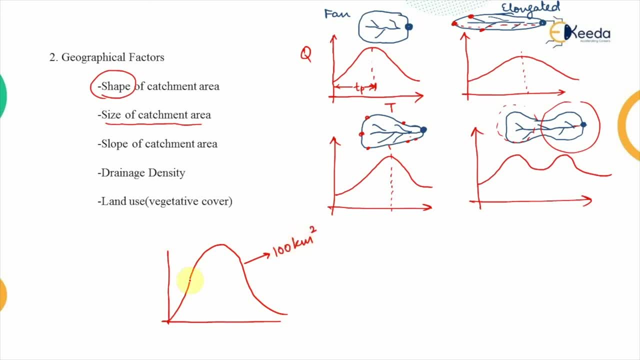 having an area of 100 square kilometers and corresponding to this, if we are having an area of 20 square kilometers, so the correspondingly the curve that we will be getting that will be somewhat like this or even below this. that means the correspondingly the discharge that 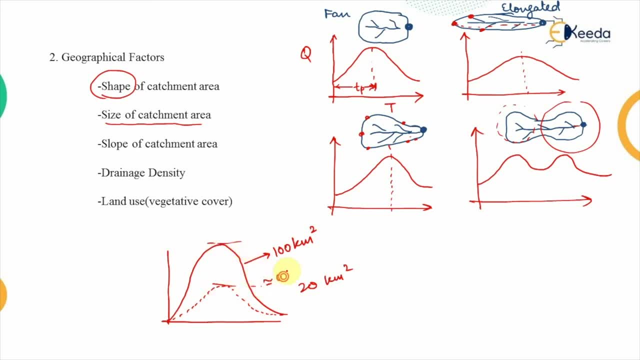 we will be getting. that will be roughly 0.2 times of the peak discharge that was obtained for the 100 square kilometer. that will be the impact of the size of the catchment area, Then the slope of the catchment area. so the slope of the catchment area if that is higher. 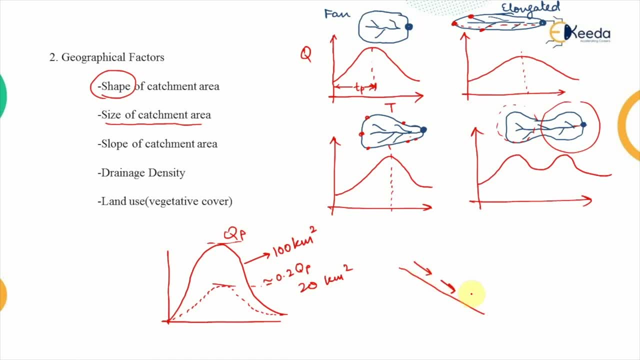 if that is very steep, then the contribution of the runoff towards the outlet point that will be quicker. if that is steep. On the other hand, if that slope is almost flatter, then the contribution or the speed with which the runoff will be moving that will be slower and because of that the 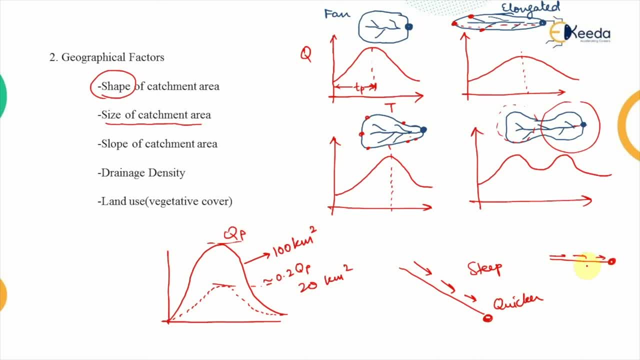 contribution towards the outlet point will also be slower. So that is the impact of the runoff, With the help of the slope of the catchment area. the next factor is the drainage density, and that is a ratio of the channel length to the drainage area. that means, in a particular 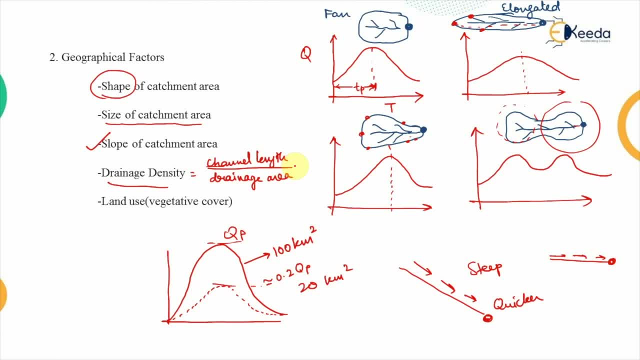 catchment area, how much length of the channels are available. that is representing the density drainage. representing the density of the drainage, that means to take the water from the entire catchment area. how many channels are available? if the lesser channels are available, that means it would take the huge amount of time to reach to the outlet point and, on the other hand, 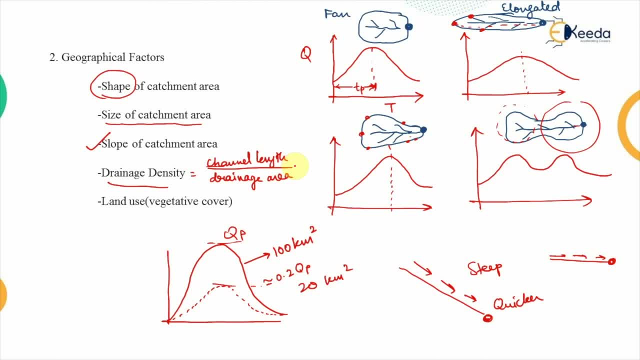 if we are having more number of channels, then the contribution towards the outlet point will be quicker and will be more, and therefore for the more drainage density we will be getting the higher peak and the peak will be obtained at the quicker point of time. Then the last point is the land use or the vegetative cover. so this act as the hindrance.